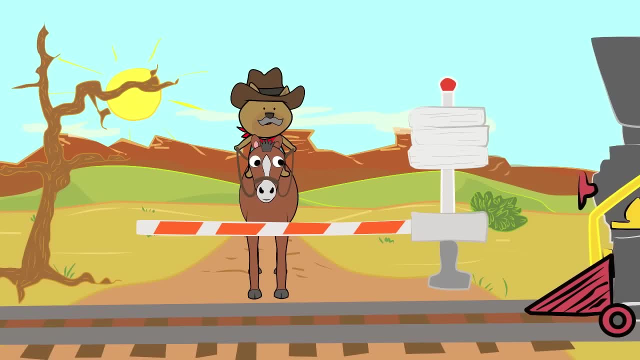 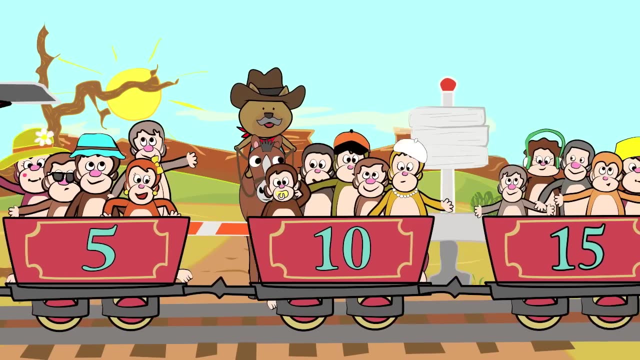 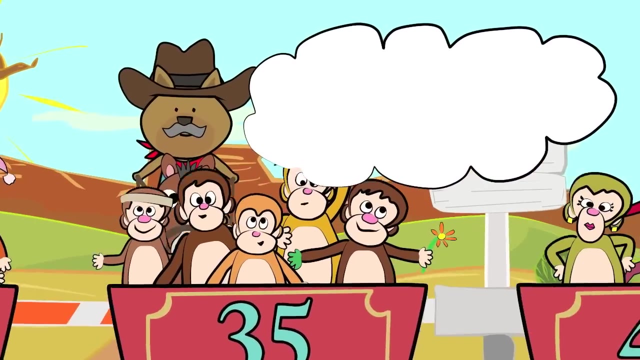 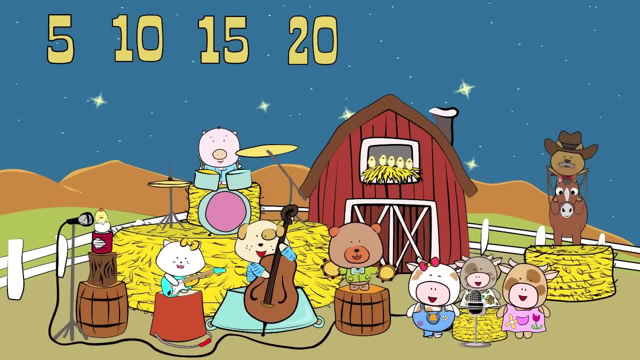 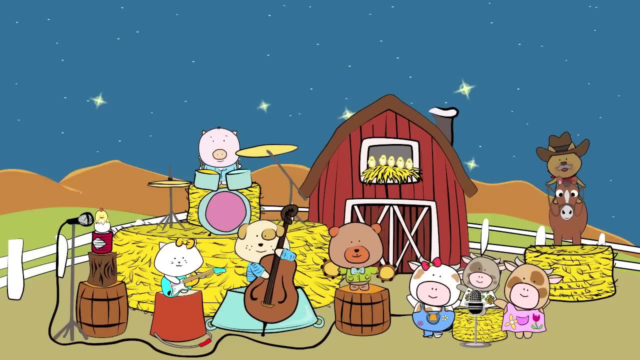 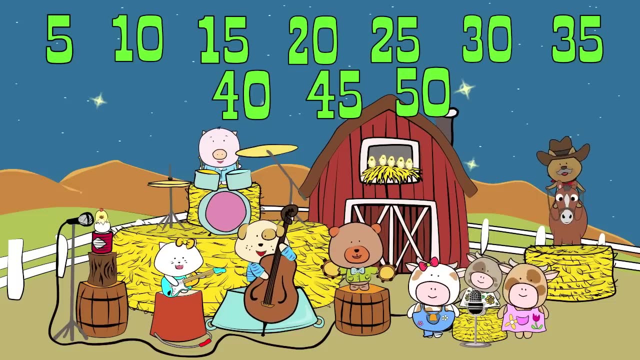 5,, 10,, 15,, 20,, 25,, 30,, 35,, 40,, 40, 550. Count by 5: 5,, 10,, 15,, 20,, 25,, 30,, 35,, 40,, 45, 50. Thanks for watching. 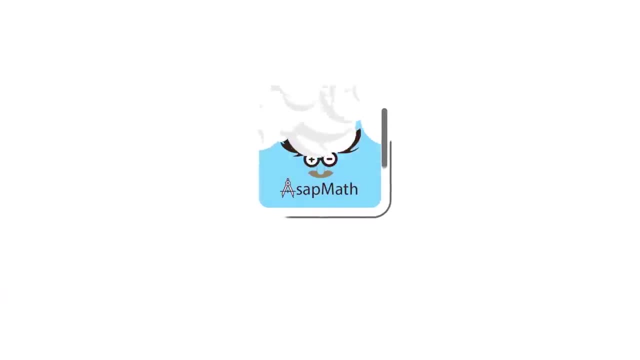 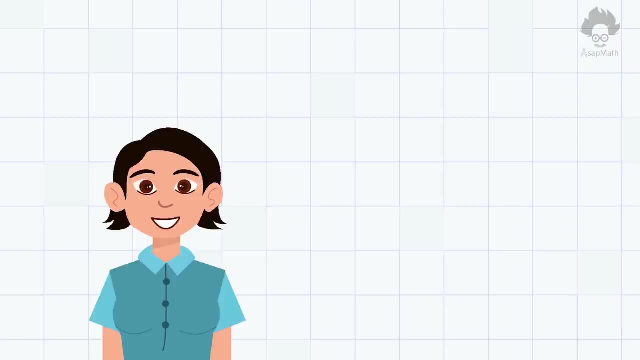 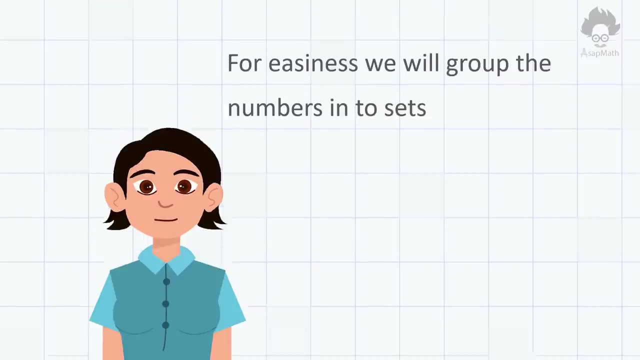 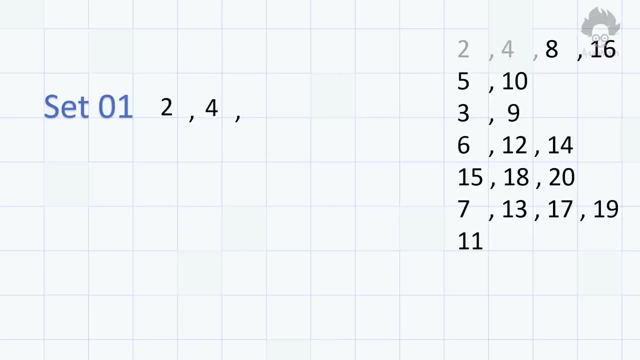 Hello everyone. in this video we are going to talk about divisibility rules of numbers between 2 and 20.. For easiness, we will group the numbers into different sets. Set 1 consists of numbers 2,, 4,, 8 and 16.. This set exhibits a similarity: all numbers are powers of 2.. 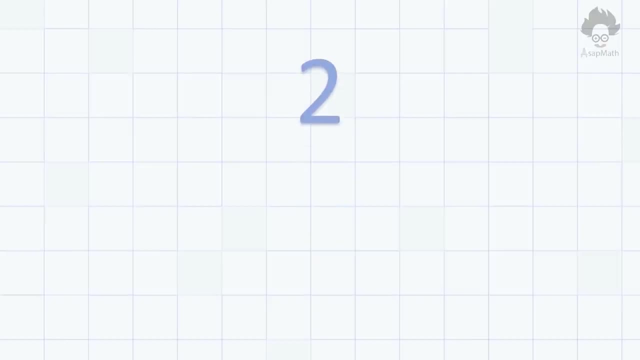 Moving on to first set. First number is number 2.. If the last digit of a number is divisible by 2, then the whole number is divisible by 2.. Let's consider a few examples Here. last digit is considered. 2 is multiple of 2.. So 32 is divisible by 2..